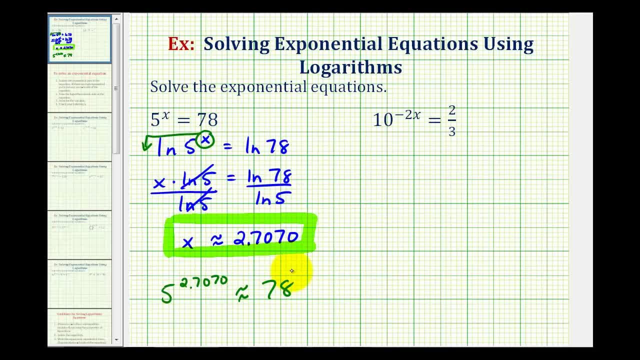 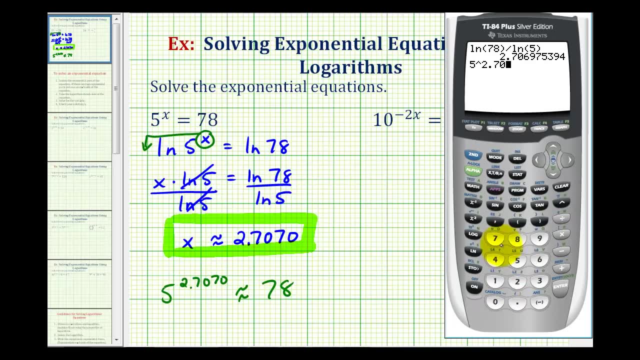 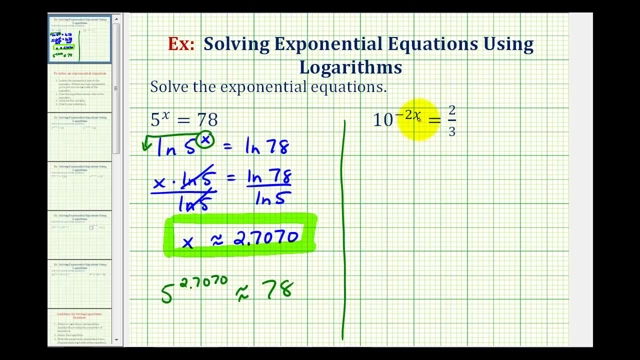 should be approximately equal to seventy-eight. So let's go ahead and check this. Notice how it is almost seventy-eight. It's a little bit larger than seventy-eight because we did round up, but this does verify our solution. Let's take a look at our second example. Here we have ten raised to the power of negative two x. 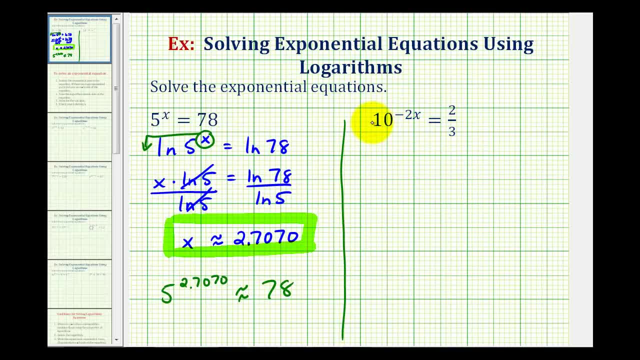 equals two thirds. The exponential part is already isolated on the left side of the equation. So now we'll take either the common log or natural log of both sides of the equation, And because here we have base ten, I'm going to take the common log of both sides. So we'll have the log. 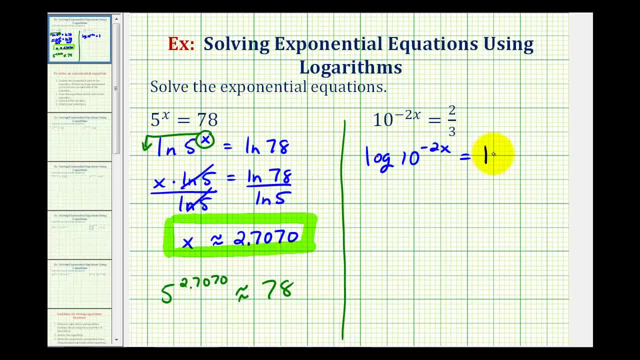 of ten raised to the power of negative two x equals log two thirds. And now we can apply the power property of logarithms to move this exponent of negative two x to the front, So we'd have negative two x times log ten equals log two thirds. 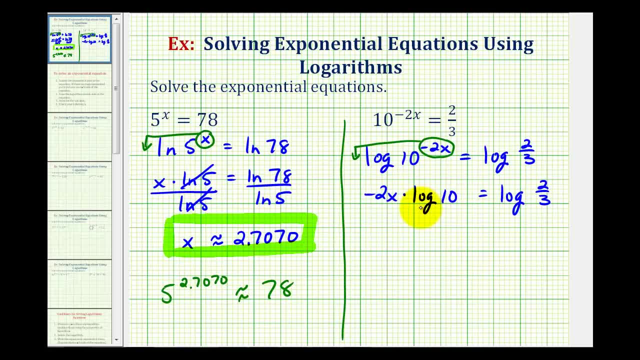 Now, the reason I wanted to use common log on this example was because the common log of ten is equal to one, So we could just drop this, but I'm going to go ahead and leave it in, just in case we didn't recognize that. 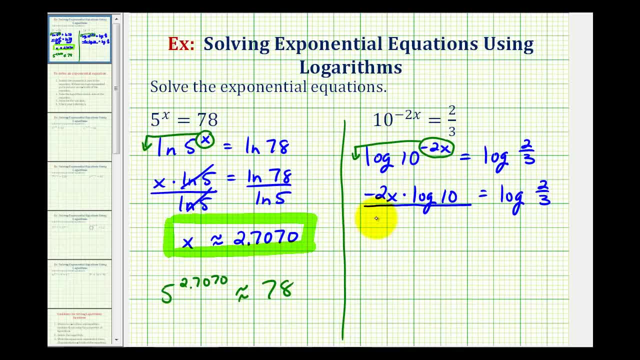 So now to solve for x, we'd have to divide both sides of the equation by negative two, log ten. Notice on the left side: negative two over negative two simplifies to one as well as log ten over log ten. So x equals negative two over negative two, simplifies to one as well as log ten over. 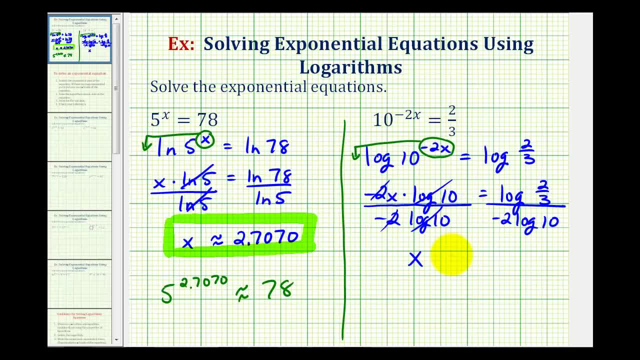 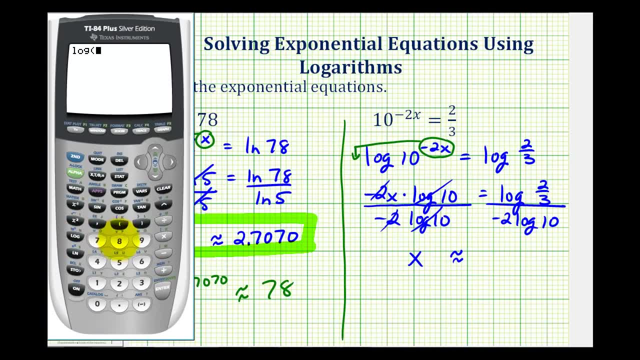 log ten. So x is going to be equal to this quotient here, which we will have to round again. So let's go back to the calculator. and now we're using the common log. so we'll press log two thirds for the numerator two divided by, three divided by. we need an open parenthesis. 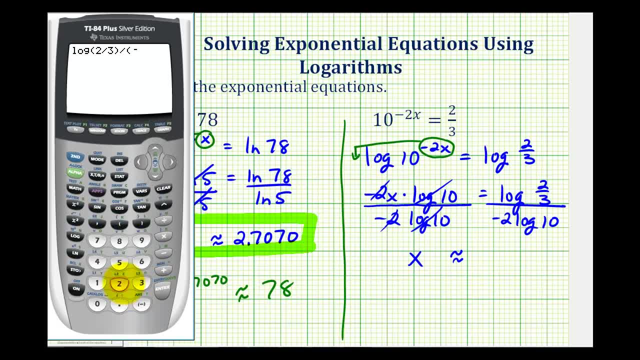 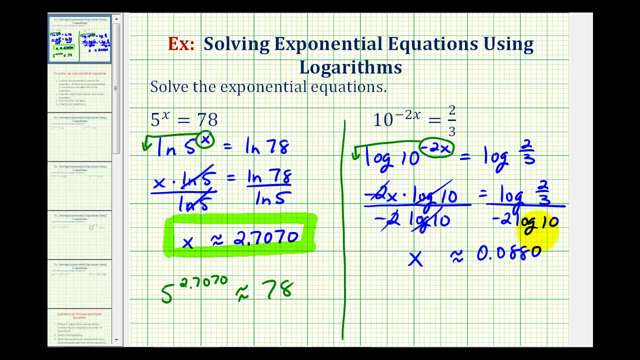 for the entire denominator negative two. of course, log ten is one, but I'll go ahead and type it in. So we have a closed parenthesis for the log and for the denominator And enter. So x is approximately point zero, eight eight zero.